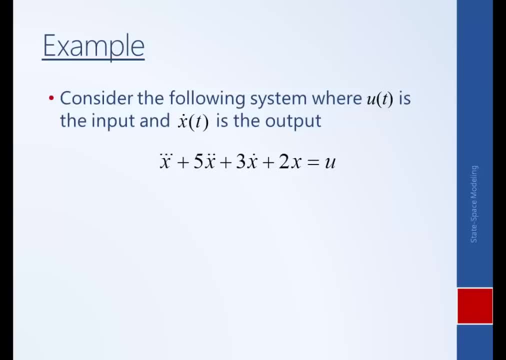 So here is a model of a physical system, a dynamic system, And if we look at it, we have a third-order differential equation modeling the system. By definition, this is not in state-space form. In order to be in state-space form, we need to model the system as a series of first-order differential equations. 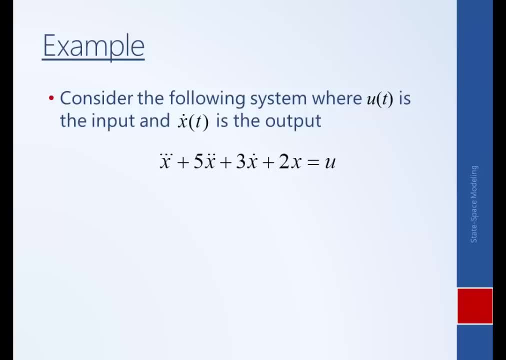 Here the highest derivative is third-order. Therefore, one way to put a differential equation model into transfer function form is to simply do a change of variables. So here we have a third-order differential equation. By choosing this new set of variables, we can rearrange this as three first-order differential equations. 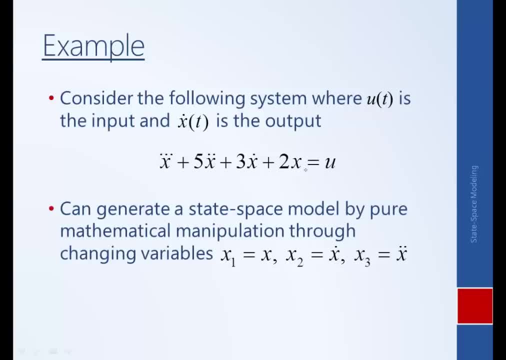 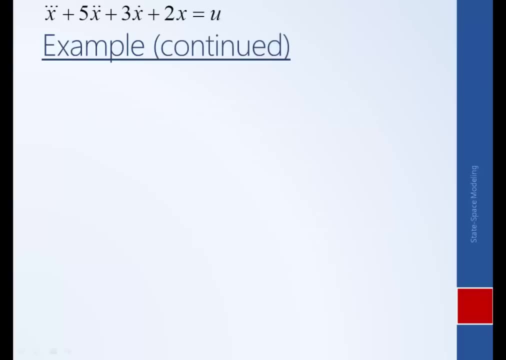 So we have a variable for the lowest derivative, the zeroth derivative, the first and the second- The highest derivative- does not need its own state variable. So here we repeat the original differential equation. We're going to do this change of variables in order to put it into state-space form. 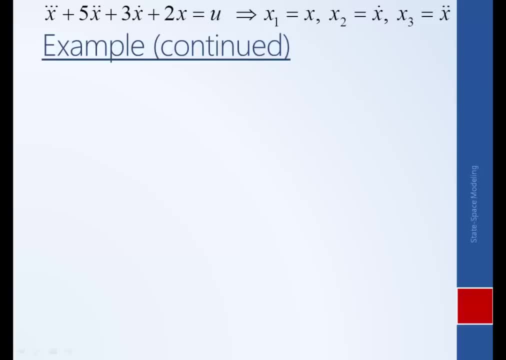 For each of the state variables we're going to have a single differential equation. So our first state variable, x1, we're going to have a differential equation for it. x2 will have its own differential equation And x3 will also have its own differential equation. 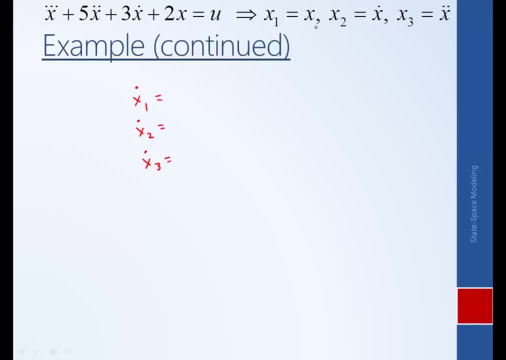 Examining this, x1 is equal to x. Therefore, its first derivative is x-dot. In terms of the state variables that we've defined, x-dot also happens to be equal to x2.. So there's our first differential equation. Similarly, x2-dot. since x2 is equal to x-dot, x2-dot will simply be x-double-dot. 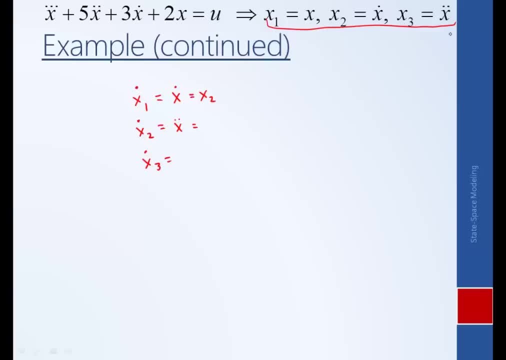 Which happens to be equal to x3.. And then, finally, x3, its first derivative is x-triple-dot. We don't have a state variable equal to x-triple-dot, but we do have the original differential equation which we can express x-triple-dot in terms of the other state variables. 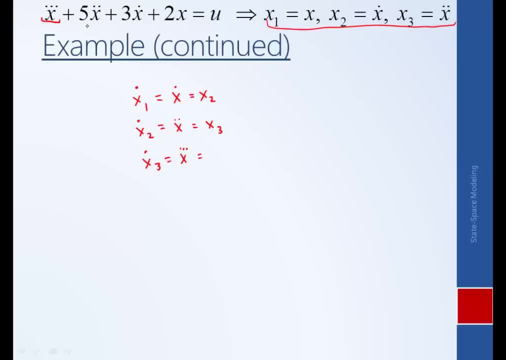 So if I subtract all of these terms to the other side, I have negative 5x-double-dot where x-double-dot is x3.. I have negative 3x-dot where x-dot is x2.. And I have negative 2x where x is x1.. 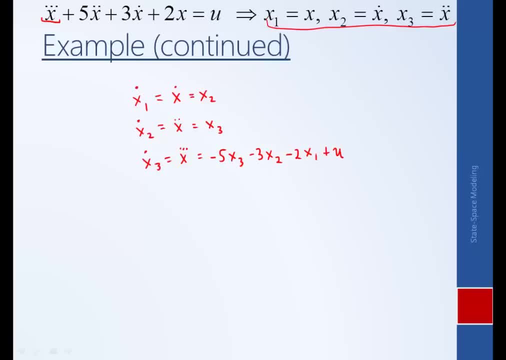 And then I already had a u on the other side. And so what we've done is we've taken our original third order differential equation and we've taken our original third order differential equation, and we've taken our original third order differential equation. 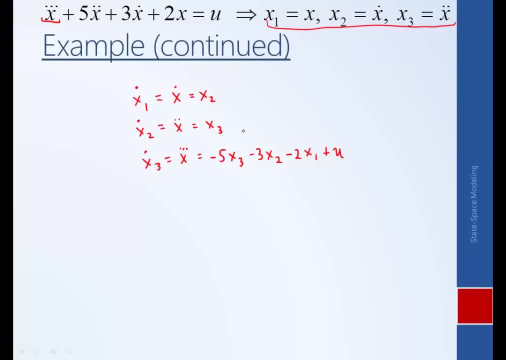 equation model and written it as three first-order differential equations. We define these three equations as our state equations. State-space form also includes an output equation or a series of output equations. What defines the output is sort of an engineering decision. You know, it depends what we're. 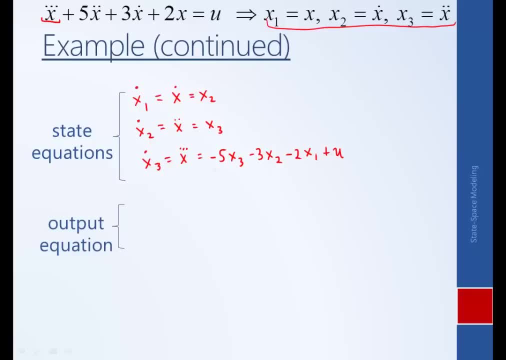 trying to control. it depends what we're trying to analyze. So position could be the output, velocity could be the output. both could be the outputs. So let's say arbitrarily that in this case x dot is the output. That just means that our 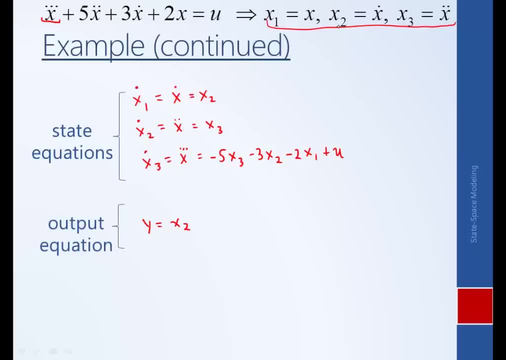 output is x2 because x dot is equal to x2.. This is something that you'll have to be told or you'll have to decide based on what it is you're trying to accomplish. So, looking at this, this is a complete state-space model and 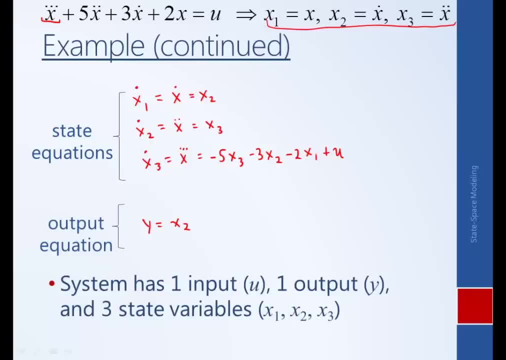 this is a complete state-space model. So, looking at this, this is a complete state-space model and of the original differential equation. this particular system has one input, u, it has one output, y, and it has three state variables, being the x1,, x2, and x3.. 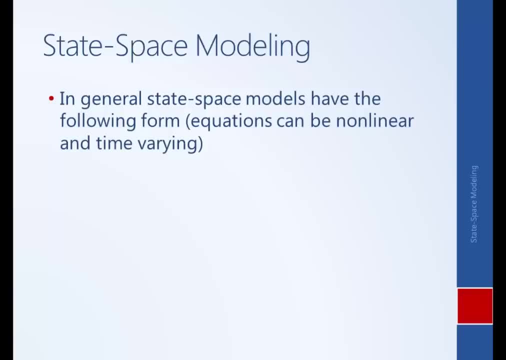 In general, state-space models have the following form: Okay, so we have a derivative for each of the state variables and each of those derivatives is a function of the other state variables and all of the inputs where there could be more than one input. You'll notice that these are all. 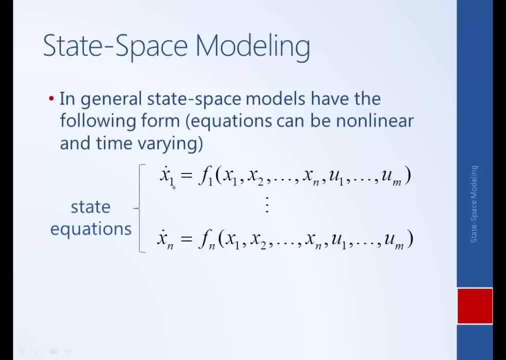 first-order differential equations. They have a single first-order derivative, being a function of non-derivatives, of only state variables and inputs. One thing that's interesting to note is that these functions can be nonlinear and they can be time-varying, So the function itself could be. 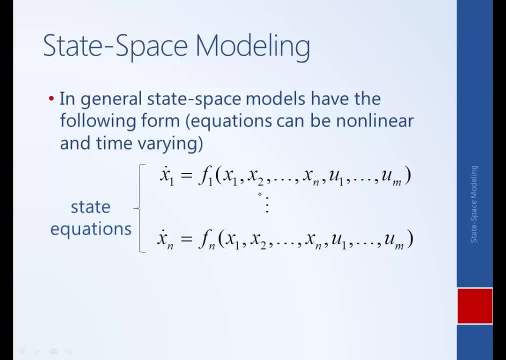 a state variable. squared, it could be the sign of a state variable, etc. Furthermore, the coefficients don't necessarily need to be constant. They can change with time. So this is a very general format that's applicable to basically any sort of dynamic system. Similarly, we have output equations, which 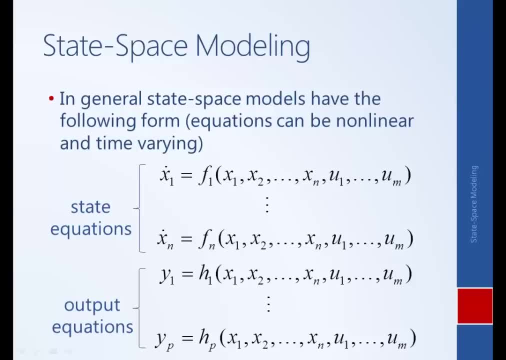 are algebraic equations. There are no derivatives in the output equations. In this case we have p outputs And each output is a function of the state variables and the inputs. So this is the most general form of a state-space model where it could be. 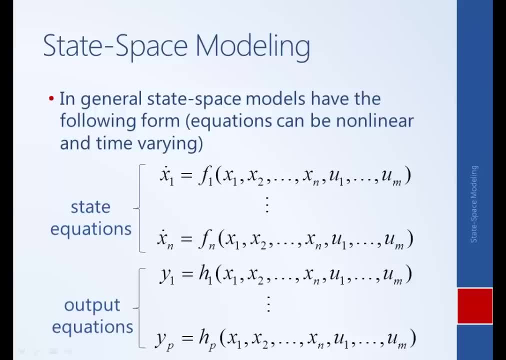 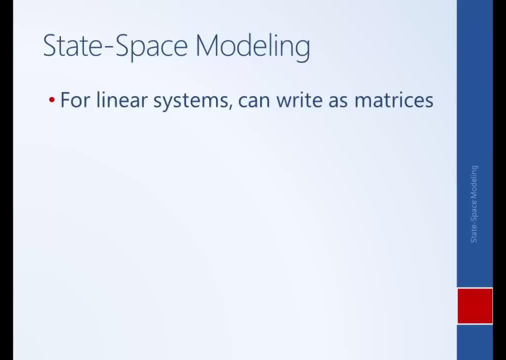 linear or nonlinear, varying or time-varying. If it turns out that our system of equations are linear, then we can rewrite them as matrices And this is the general form. So we have a vector of the derivatives, of all of the state variables. We have a 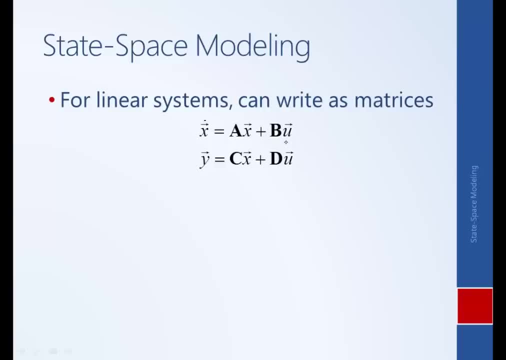 matrix A multiplying the vector of state variables, We have a matrix B multiplying the input variables. So this matrix equation constitutes all of the state equations. And then we have a second matrix equation for all of the output equations, where we have a vector of outputs equal to a C matrix times a. 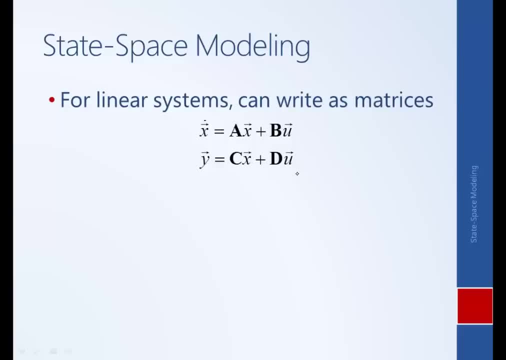 vector of state variables plus a D matrix multiplying a vector of inputs. So, if we consider our previous example, here are the state equations, Here is the output equation. We can rewrite this in matrix form because these are linear equations. So specifically, we'll have a vector of 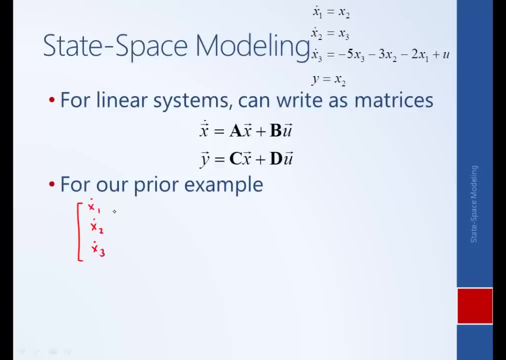 derivatives of our state variables x1 dot, x2 dot and x3 dot. We'll have an A matrix multiplying a vector of state variables. We'll have a B matrix multiplying a vector of inputs. In this case, we have only a single input, a scalar input. 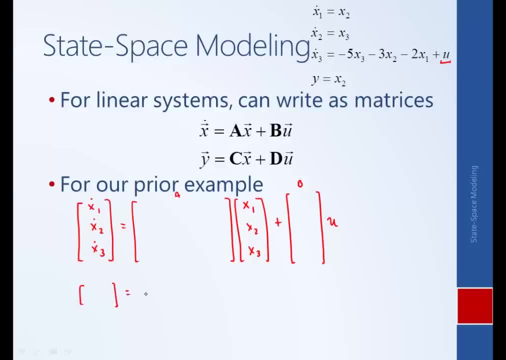 And then we'll also have our output equations. We'll have a vector of outputs- In this case, we have only a single output, a scalar. We'll have a C matrix multiplying a vector of state variables And we'll have a D matrix multiplying our input vector, which in 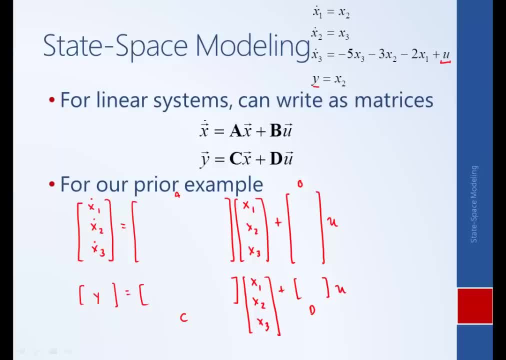 this case has only one element. So, looking at the first part, with our A matrix, the first row of the A matrix is going to represent our first state equation. so x1 dot is equal to x2.. So that means that the first row of our A matrix is going to be zero. one but zero. 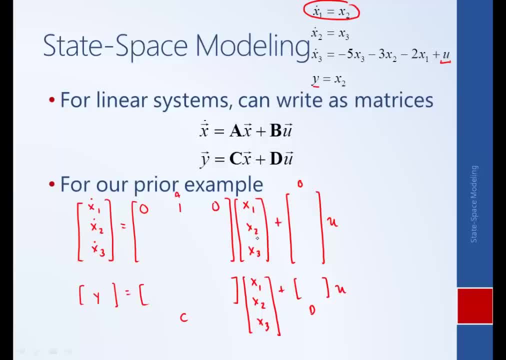 If we took this row, multiplied it by that column, we would get zero times x1 plus one times the x1.. x2 plus 0 times x3, meaning x1 dot is equal to x2, just as we have here Since. 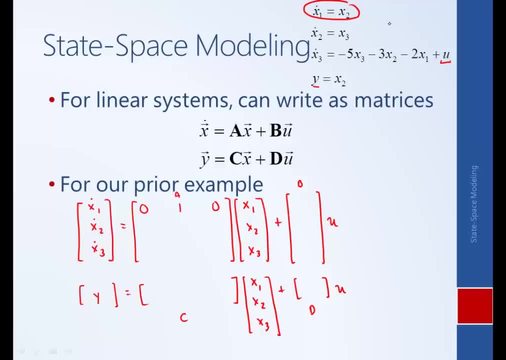 the first equation is not a function of the input u. that row of the B matrix is just 0.. The second row represents what x2 dot is equal to. so it's 0 times x1,, 0 times x2,, 1 times x3, and 0 times u. And then the last row constitutes the 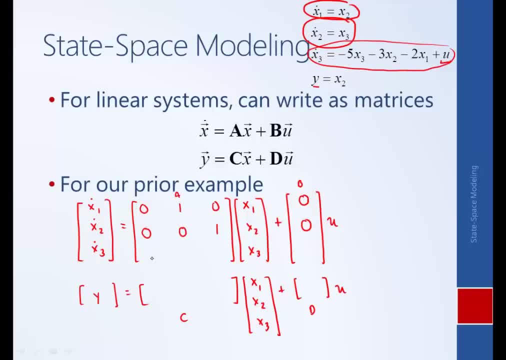 equation for x3 dot. So multiplying x1 is a negative 2,, multiplying x2 is a negative 3, multiplying x3 is a negative 5, and multiplying u is 1.. So there, we've filled out our state equations. We have an A matrix and a B matrix.